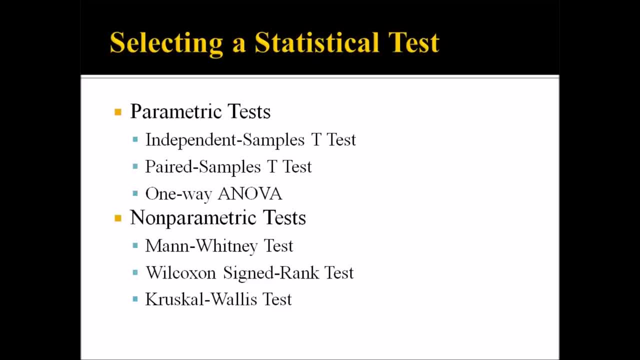 The choice between using a parametric test and a non-parametric test comes down to analyzing the data and determining if it's more appropriate, if it meets the guidelines for parametric testing, Non-parametric testing, and sometimes making this distinction is not easy. 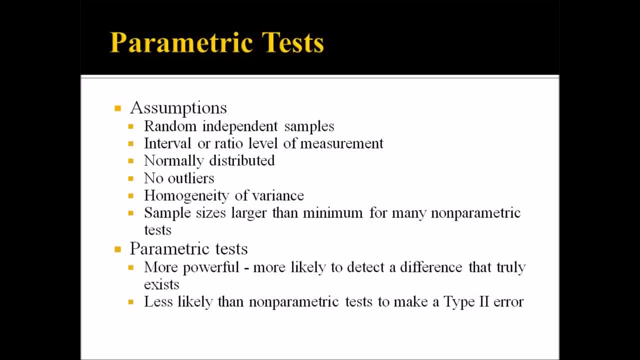 So let's take a look at the parametric tests. Generally speaking, in counseling research, we always look to parametric tests first. So if we're analyzing data and we're trying to decide what type of test to use, we're going to evaluate that data, analyze that data in terms of can it be used for parametric? 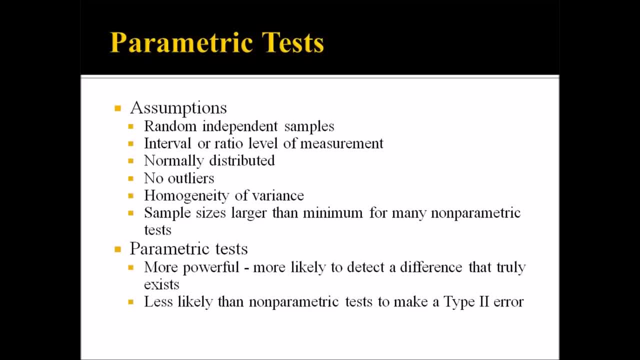 testing And if it cannot be used for parametric testing, we will use non-parametric tests. So the assumptions for parametric tests would be examined first, And different parametric tests have different assumptions. but here are some fairly common assumptions. So, for example, let's say you have a test called IC. 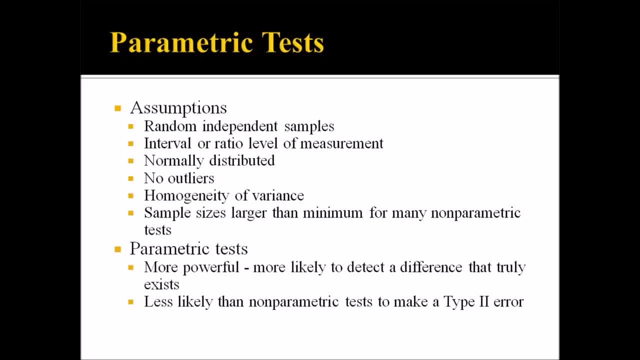 You've got an IC. that's an IC for parametric tests. You need random independent samples, interval or ratio level of measurement. So no nominal or ordinal level variables, only interval or ratio. SPSS refers to both interval and ratio together as scale. 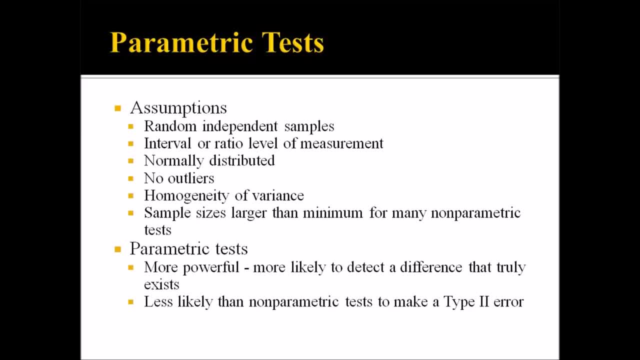 So they have nominal, ordinal and scale. So in the case of using SPSS, you'd be looking for a scale level measurement. The data must be normally distributed. Many parametric tests do not accept outliers. Many have the assumption of homogeneity of variance. 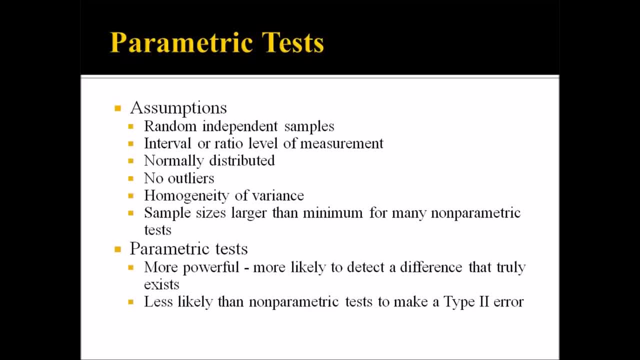 And, in general, the sample sizes need to be larger for parametric tests as compared to what would be the minimum for many non-parametric tests. Parametric tests are generally preferred because they are more powerful. This is a very specific term. I'm referring to statistical power, meaning these tests are more likely to detect a difference. 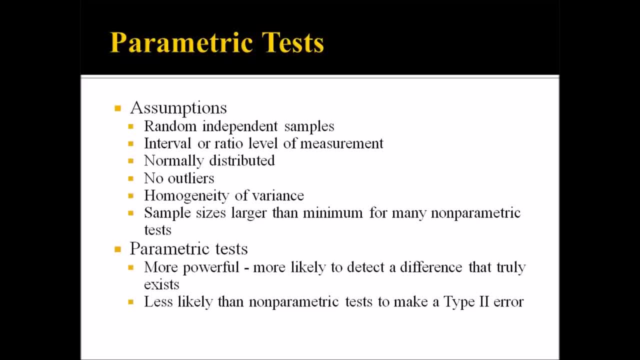 that truly matters. Parametric tests are less likely than non-parametric tests to make a Type II error. A Type II error is when we fail to reject the null hypothesis when in fact the null hypothesis was false. A Type I error is when we reject the null hypothesis but it was in fact true. 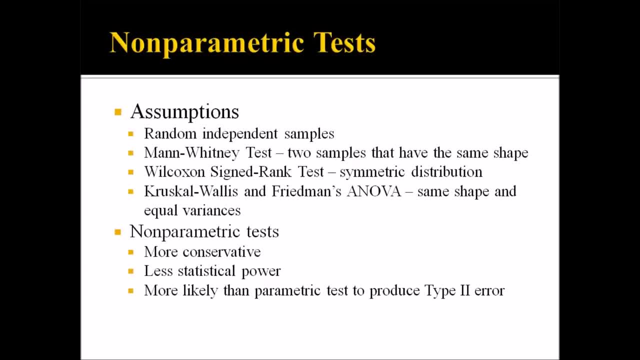 Moving on to non-parametric tests, As I mentioned before, we usually take a look at the assumptions for parametric tests first, and if the assumptions aren't met, we use the corresponding non-parametric test. And even though non-parametric tests do not have the same number of assumptions, they're 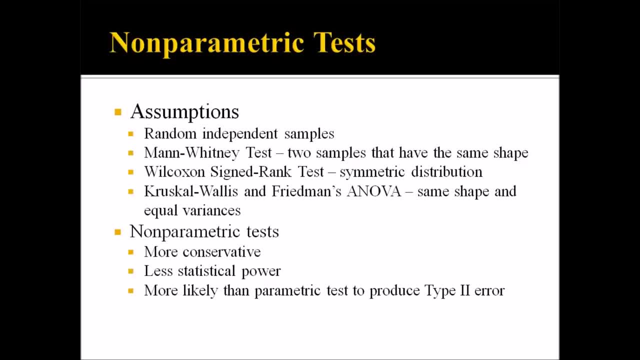 not as rigid in terms of the assumptions the data have to meet. there are still assumptions with non-parametric tests. The first assumption- random independent samples- is that the data is not as rigid as the assumptions are. This is one of the common assumptions for parametric tests as well. 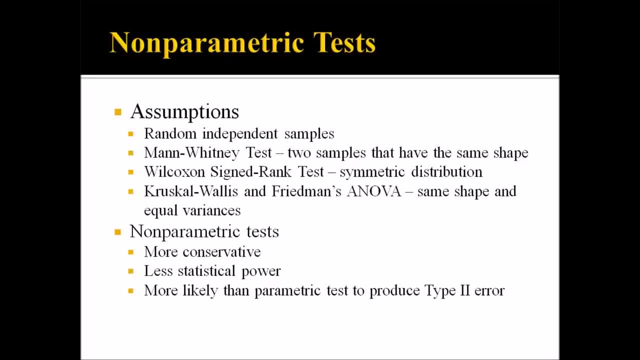 And then looking at some specific non-parametric tests. the Mann-Whitney test: the two samples have to have the same shape. Wilcoxon's sign rank test requires a symmetric distribution and both the Kruskal-Wallis and Friedman's ANOVA require the same shape and equal variances. 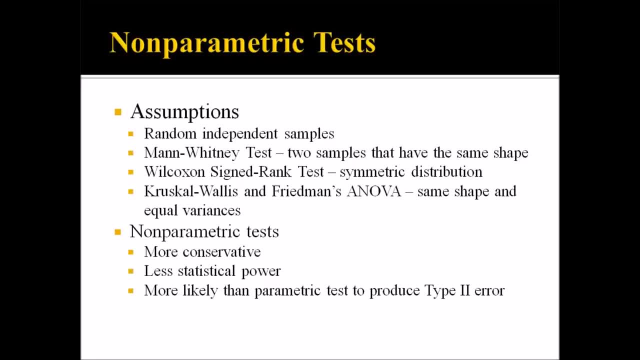 Non-parametric tests are more conservative. They have less statistical power. They are less able to detect a difference that is truly there. A non-parametric test is more likely than its corresponding parametric test to produce a type II error. So, moving on to some parametric and non-parametric tests, 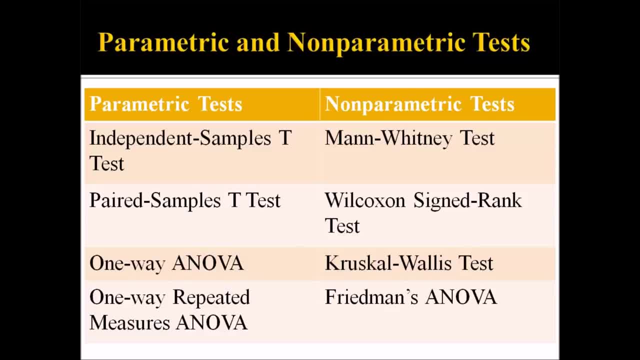 I have here in this table A parametric test on the left and some non-parametric tests on the right, And these are the corresponding non-parametric tests. So if you're looking to use an independent samples t-test and your data do not meet,